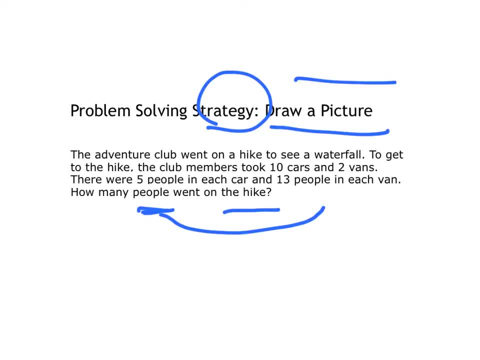 Anything that I feel will help me get this answer. I need to pick information from the problem to draw out, And I will only draw out information from the problem that will help me answer this question: how many people went on the hike? So after reading it, I know that a certain amount of people went in cars and vans. so I think I'll have to draw maybe something related to cars and vans. 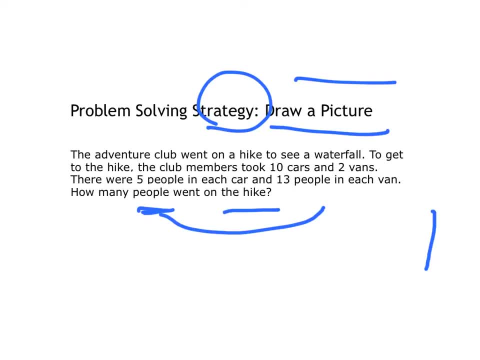 Okay, So, So, So. So It says the adventure club went on a hike to see a waterfall. To get to the hike, the club members took ten cars and two vans. I'm going to represent cars with a circle. 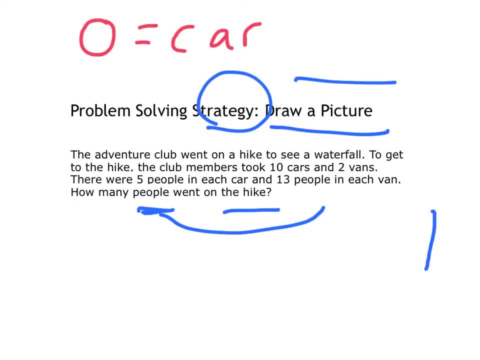 And I'll choose a different color for vans. A van will be a square, Okay, or a rectangle. Now it says there were five people in each car and thirteen people in each van. How many people went on the hike? Okay, before that it says: to get to the hike, the club members took ten cars. 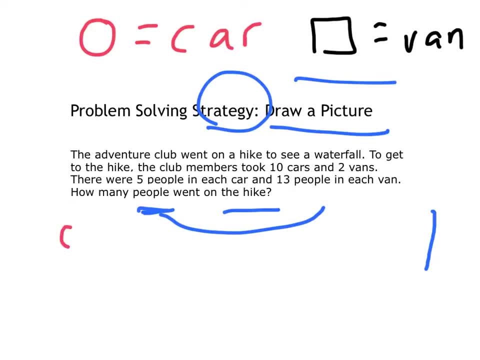 So let me draw these ten cars out. first Ten cars: One, two, three, four, five cars, six cars, seven cars, eight cars, nine cars, ten cars, And then, and they took two vans, So I'm going to draw the two vans out. 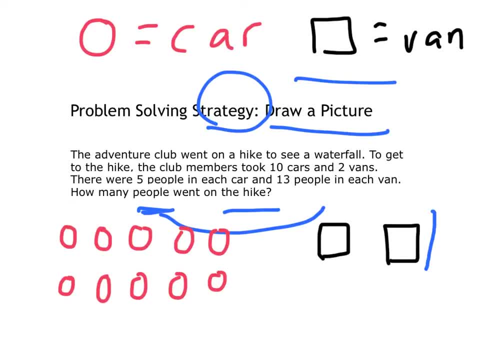 One van two van. So now I've got my ten cars and my two vans. And the next piece of information is related to solving this. It says there were five people in each car. Okay, So now I've got my ten cars and my two vans. The next piece of information is related to solving this. It says there were five people in each car. Okay. 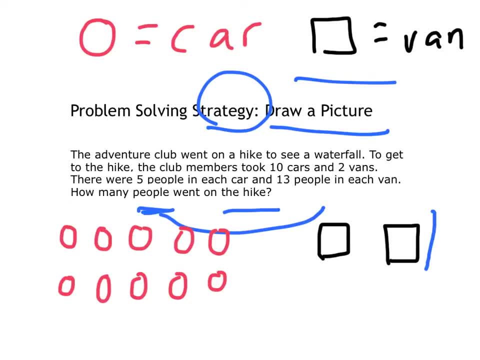 So now I've got my ten cars and my two vans. The next piece of information is related to solving this. It says there were five people in each car. Okay, So each car now is going to have five people in it. 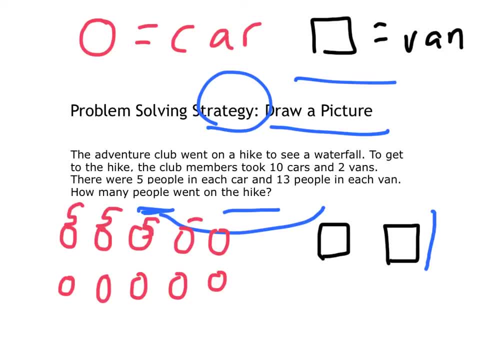 And I'm going to put a five right next to or on top of each car. And then it says there were thirteen people in each van, And in each van I'm going to put thirteen people. How many people went on the hike? 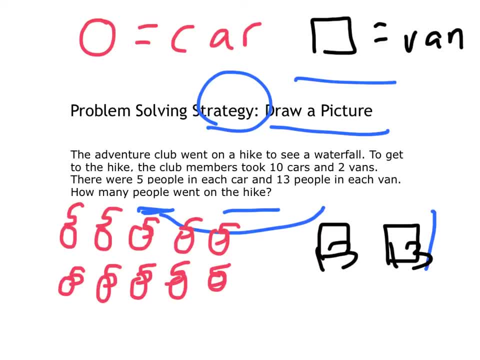 Well, this question: how many people went on the hike? there's nothing in there that indicates for me to add, but I know to add because I'm trying to find a total number of people between cars and vans. So my last step would be to add these numbers up.